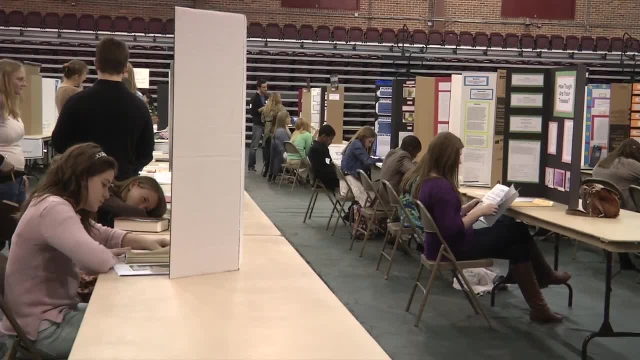 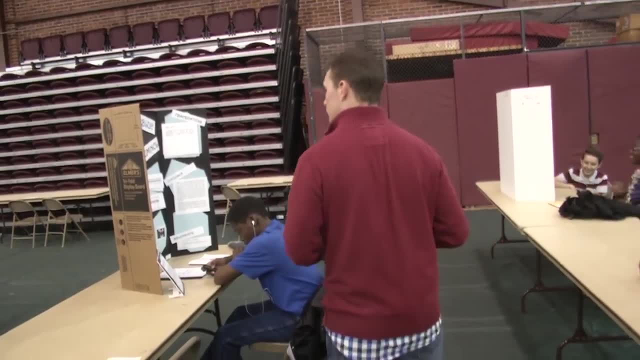 science and its applications in various contexts. So anytime we can kind of draw that out of a student, it's usually a successful experience. Well, Mallory, tell me about your project and what you learned and what you were testing and all that kind of stuff. 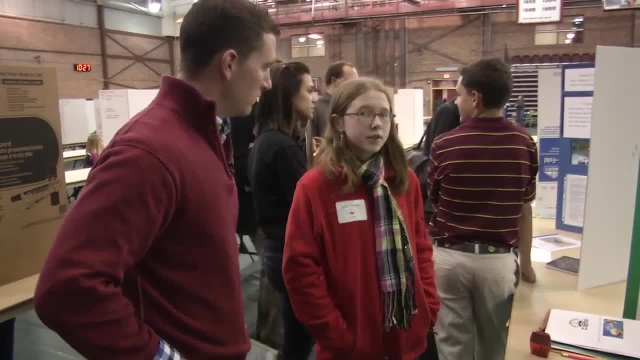 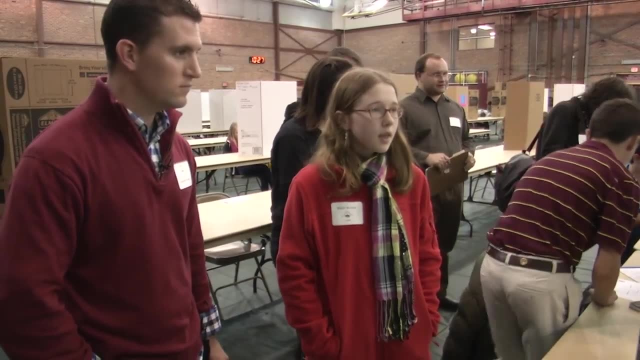 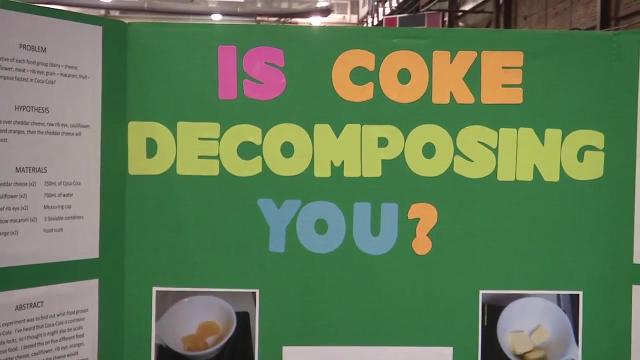 Okay, so I was testing if coca-cola would decompose certain types of food groups, and my hypothesis was that cheese would decompose out of the five food groups that I had chosen. Each day I would measure how much the food weighed and then I would put it back in the 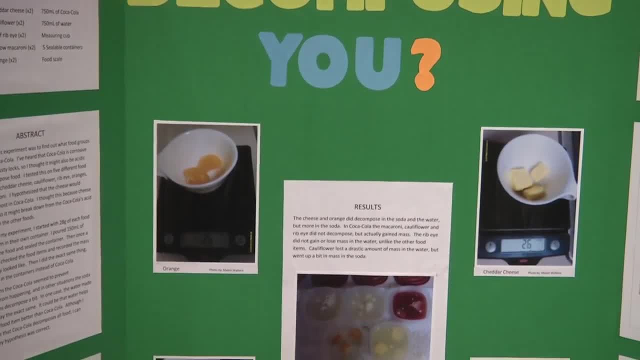 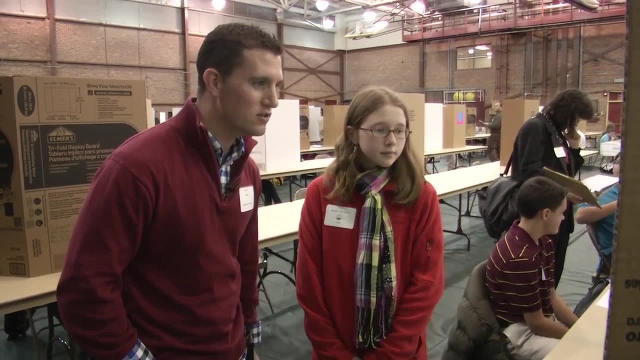 container and wait for the next day to come, And the results were kind of all across the board. but my hypothesis was correct. And tell me about your setup again. So how did you figure out what you were testing, How did you figure out what to test and how to set it up? 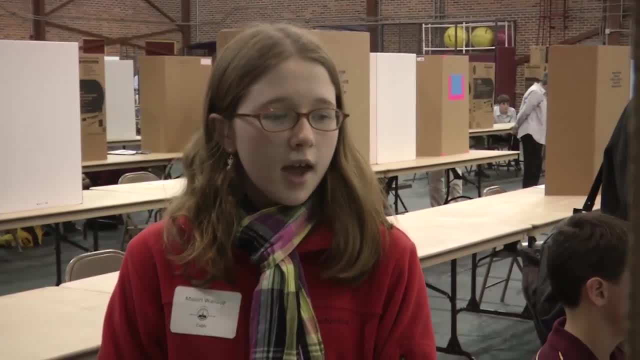 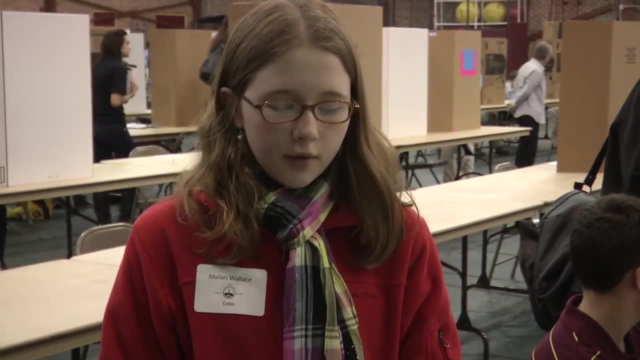 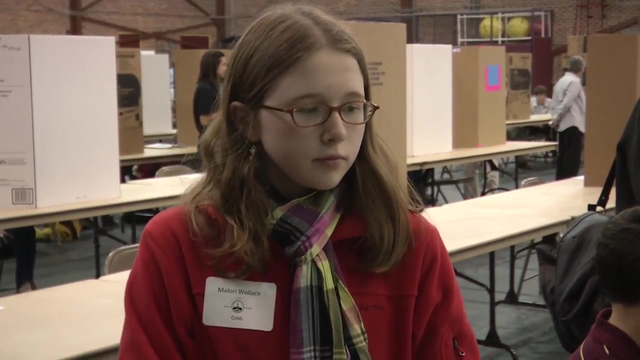 I had put them in. each one was in its own container and this one shows the water that they were in And I had. whenever I was weighing them, I used a food scale and a cylinder that I could drain the coca-cola or water out of back into the container so I could measure. 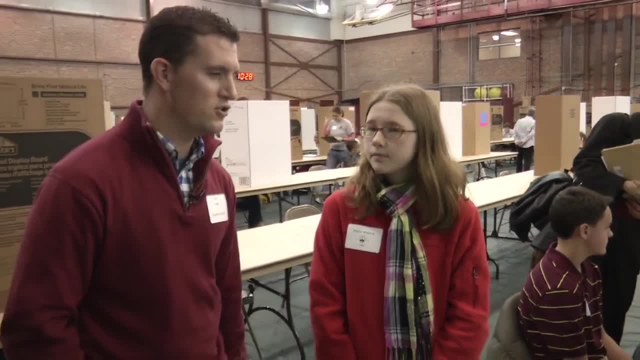 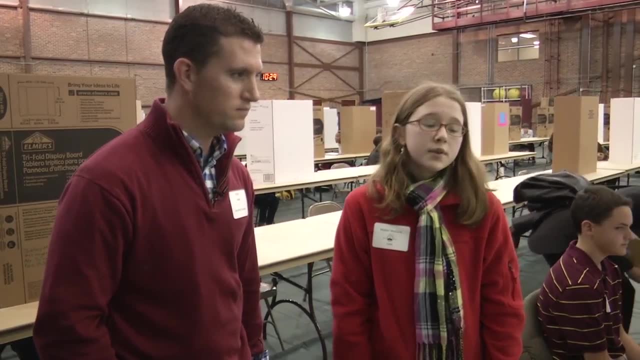 them by themselves? Okay, and tell me now. you said that you had some in water. Yes, I had some in water, Okay, And some in coca-cola. Why did you have the two different liquids? Well, the water was the base and the coca-cola was the actual thing I was testing. 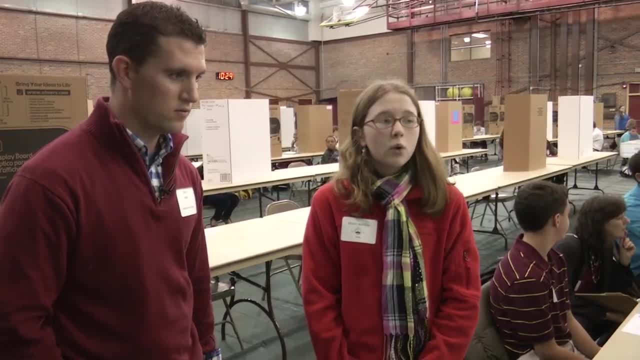 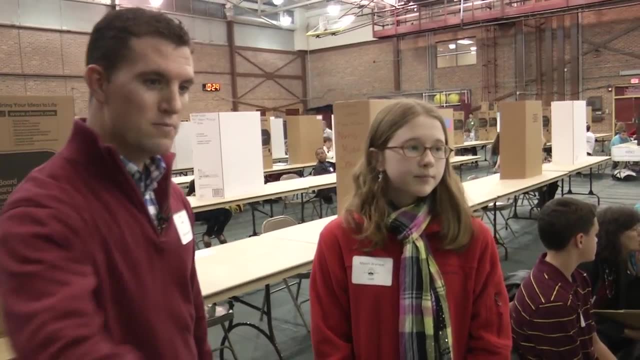 Okay, And I figured if I was testing in the coca-cola, I should probably test what it did in water also. Okay, so maybe just kind of as a point of comparison or something. Yes, Okay, excellent. Would you mind explaining to me what your graphs are showing me over? 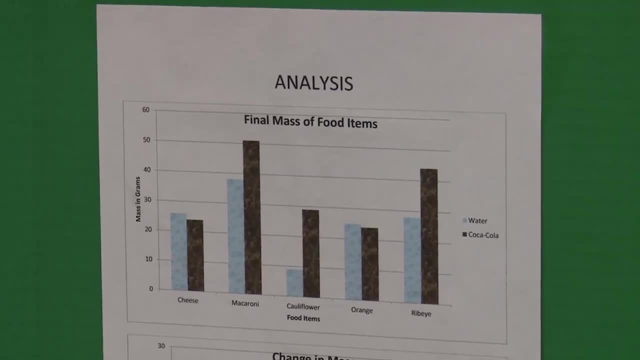 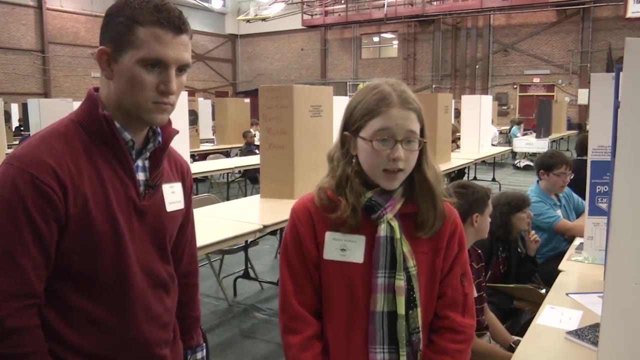 here, The final mass of the food items, shows the mass at the end of the six days, how much they weigh, How much they each measured out to be, And the change in mass is if they increased in mass, if they decreased in mass. 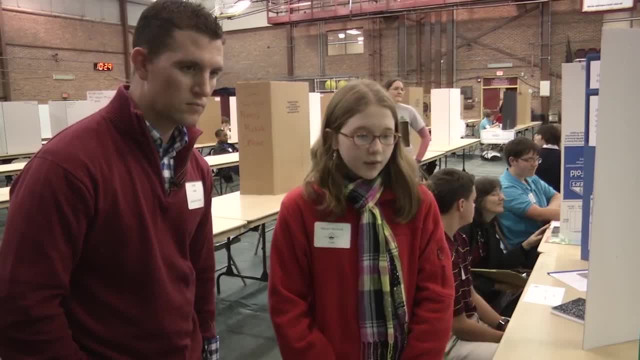 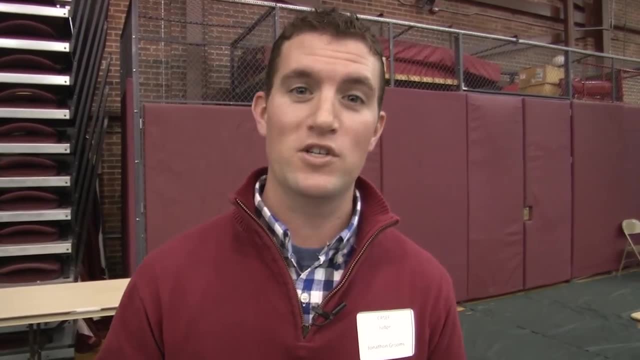 Since the results were kind of all over the place, they were very different in range. All right, Well, thank you very much for sharing your project. I appreciate it. So our last project: she had a grasp of what she was testing and she had some quality. 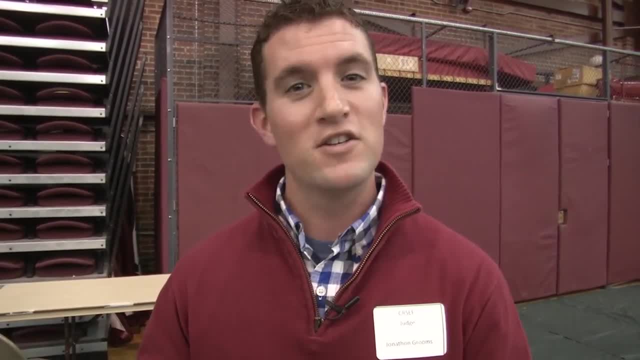 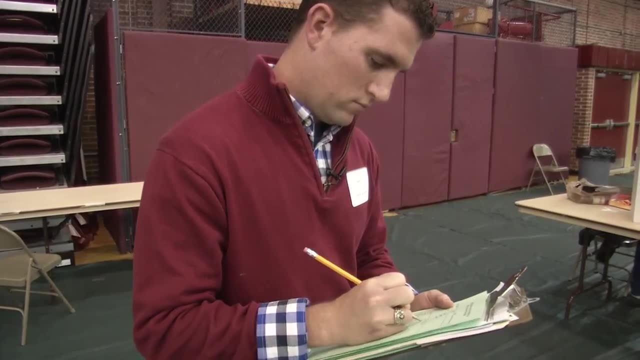 data to try and back up her results. So she was really trying to make some connections there with the data that she saw And the science that she's learned about acids and bases. So she did a really good job in trying to explain her project and what she learned. 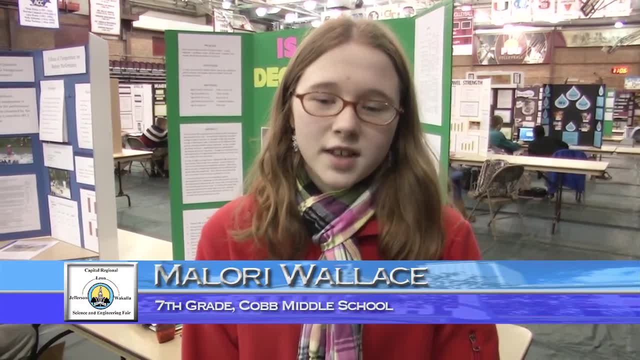 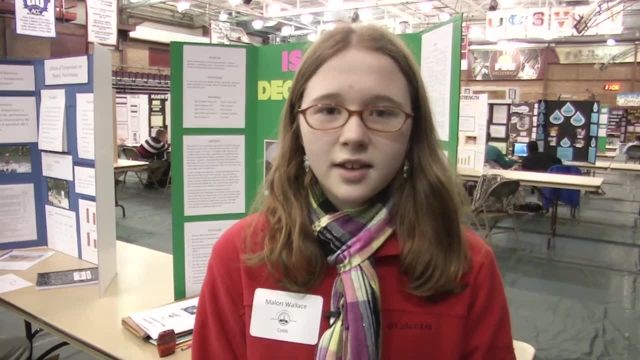 It was kind of nerve-wracking, like having all the judges come up and you just kind of tell them what you think. But after a couple of them came by it was easier and easier and I got more comfortable. And it was it started becoming better to talk to them more. 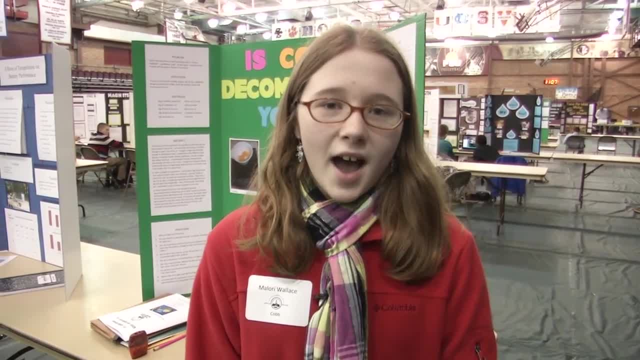 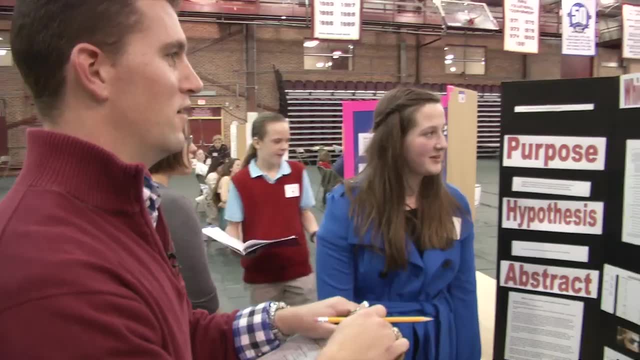 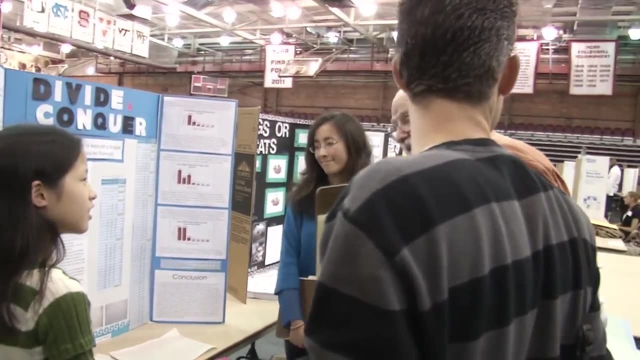 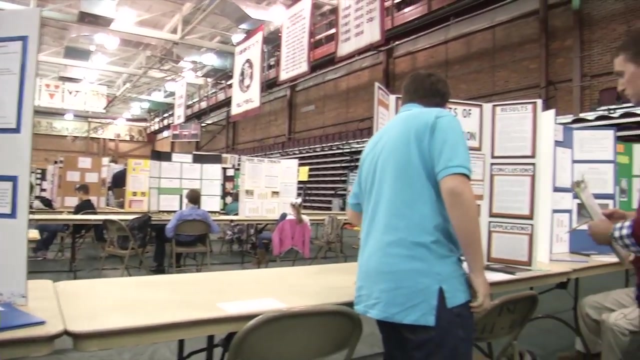 Well, I mean, of course I hope I did well, But I think I tried my best And I put everything I have out there and there's nothing more. I could give Scott Good, Jonathan Good to meet you, buddy. Tell me about your project quickly. What did you test and what did you find out? Okay, So the question was: is a battery's temperature affected performance? So my hypothesis was: if a battery's temperature is decreased, then their performance will decrease. also measured by the room time of a remote-controlled car. So we would test the batteries in dry ice, ice and room temperature. So at room temperature we got about 32 minutes, In ice we got about 25 minutes, And in dry ice we got 7 minutes. 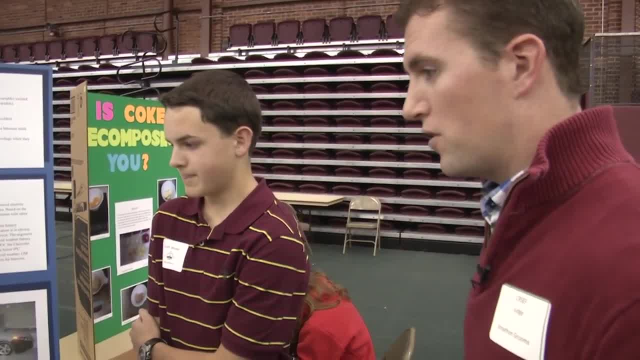 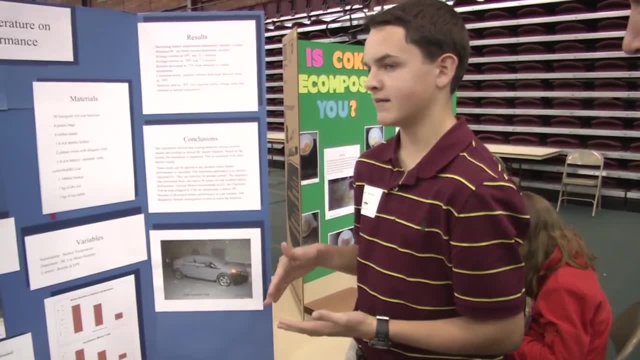 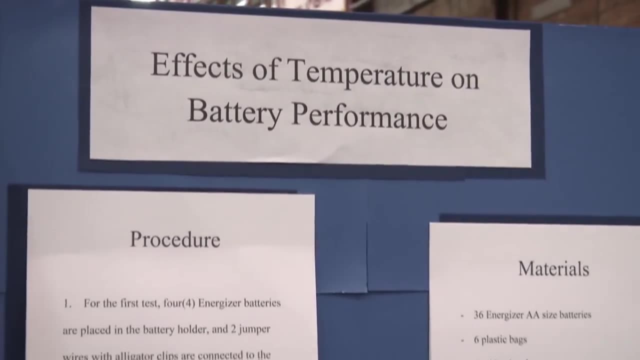 Okay, All right, So explain to me a little more the method that you used here to test the different temperatures on the battery. We put a battery pack with four Energizer batteries in it down in a plastic bag and tie it off, And then we stick. we put some dry ice in the bottom of the beaker, stick the battery. 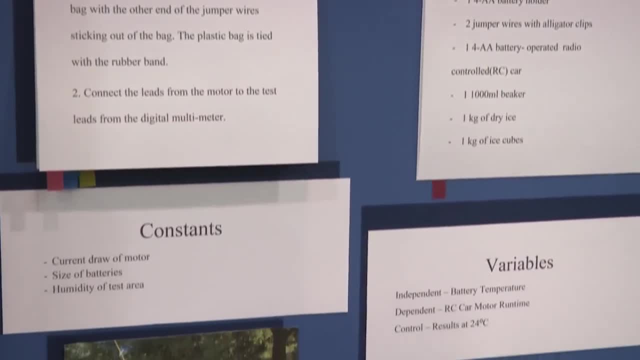 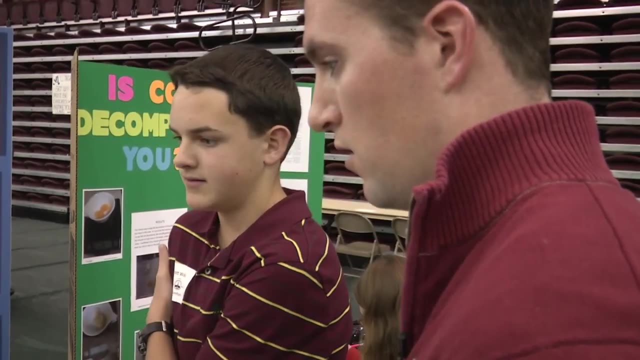 pack on it and bury it in there, And then we let it sit for 15 minutes to get cold, And then we would just use the jumper cables to hook it up to a motor. Okay, All right, And now how did you measure those temperatures? 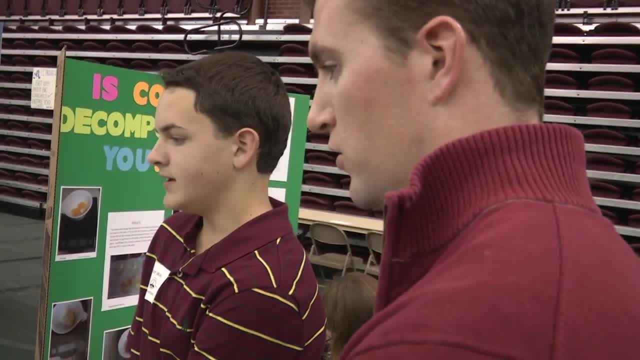 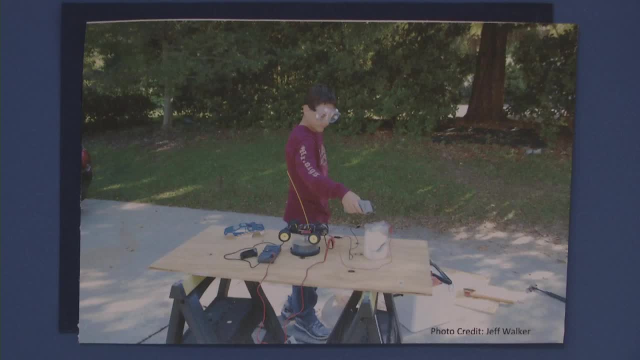 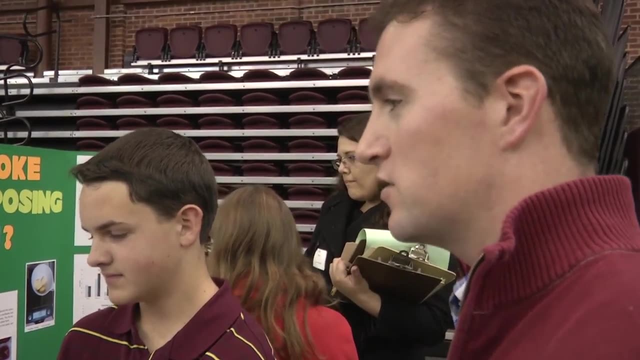 How did you make sure that the batteries were getting down to zero degrees or negative? We used a laser thermometer. We would shoot it on the ice and make sure that it was exactly Okay, All right. So if you were going to do this project again, Scott, what are some things that you might? 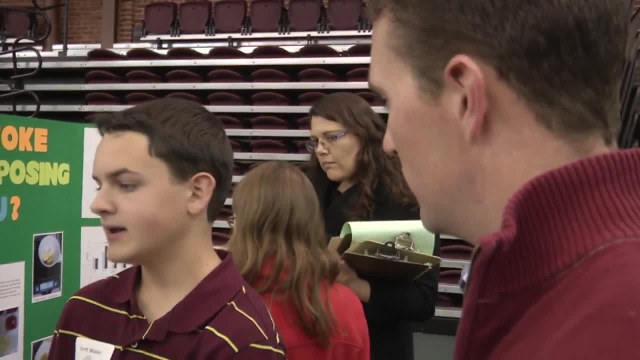 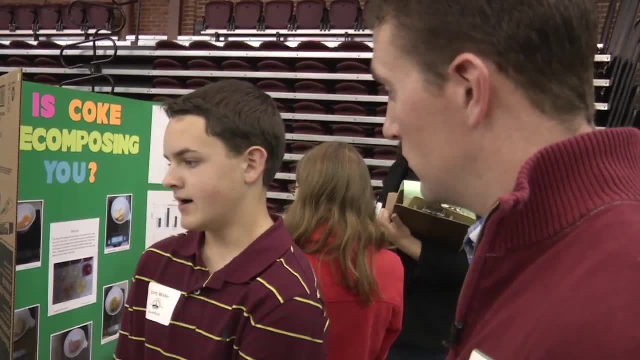 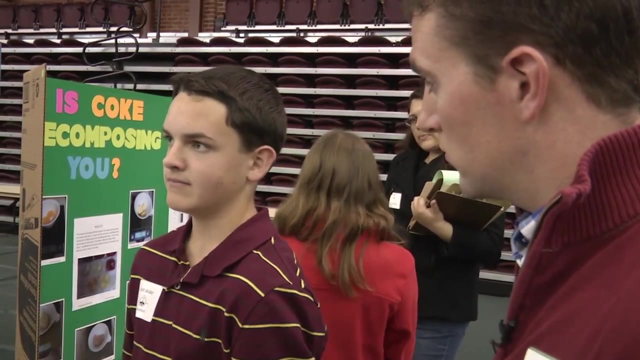 do differently or some other directions you might take. I might get a different car with a different motor in it, with a different load, and try to measure the load. We might also change the battery type. So we did a first science fair kind of.